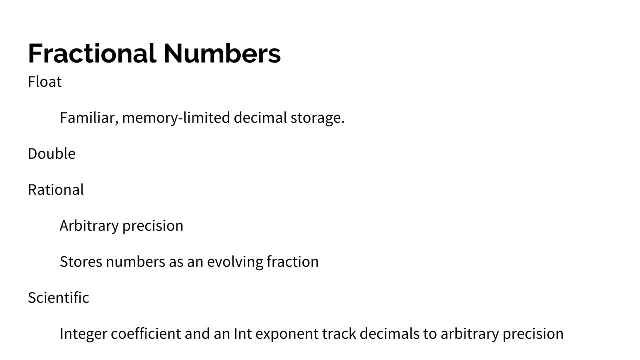 it to. The other numeric data type category is that of fractional numbers. Fractional numbers includes the familiar float and double, as well as a type called rational, which stores numbers to arbitrary precision as a fraction. For example, this type would store 1, 3rd, as 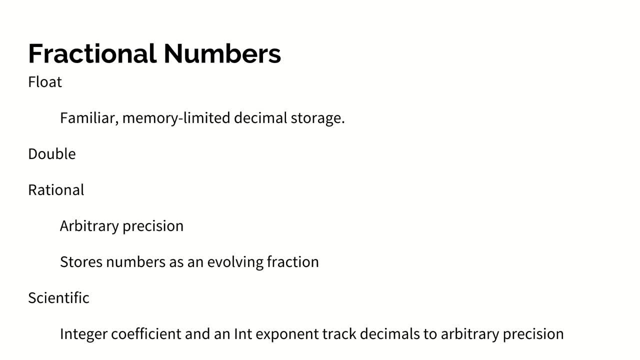 1, 3rd, The third multiplied by one-half as one-sixth. There's also the scientific data type, which stores the numbers in a scientific format, meaning there's an integer coefficient and an int exponent that tracks decimals to arbitrary precision. 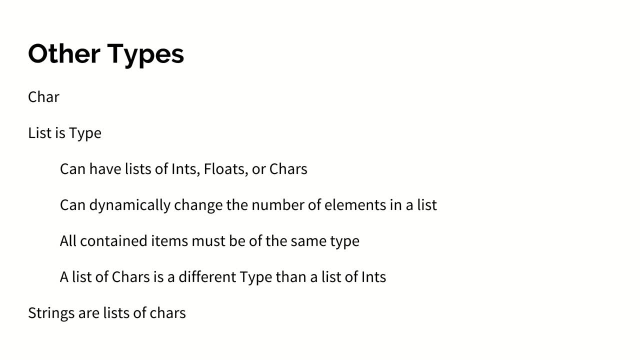 Other basic data types in Haskell include the familiar char as well as list. List is a type in Haskell. Furthermore, List is a type that is dependent on what contains. A list of ints is different than a list of integers, is different than a list of chars. However, the number of items in a list can change. 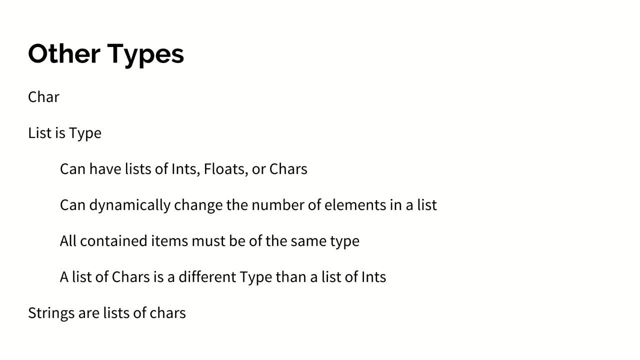 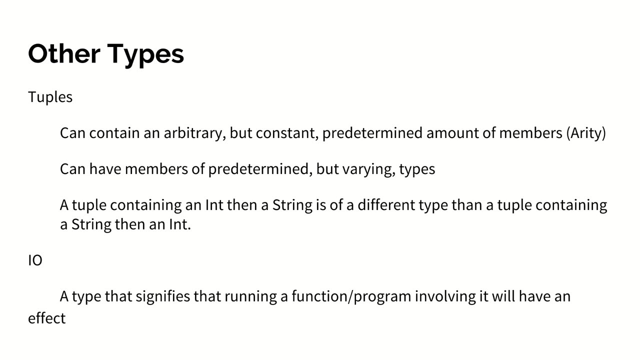 dynamically. It's just that all items contained in a list must be of the same type. Furthermore, string is just an alias for a list of chars in Haskell. Tuples are like lists in that they can contain an arbitrary amount of members. However, that arbitrary amount of members must remain constant A tuple can hold. 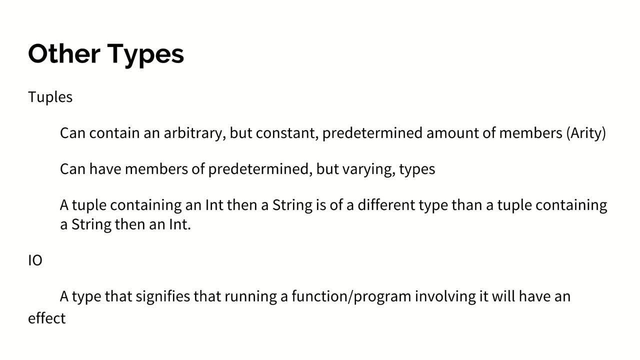 three things, but it must always have three things in it. The number of members of a tuple is predetermined. This predetermined amount of members is called erity. Also, the members of a tuple can be of different types, so you can have a. 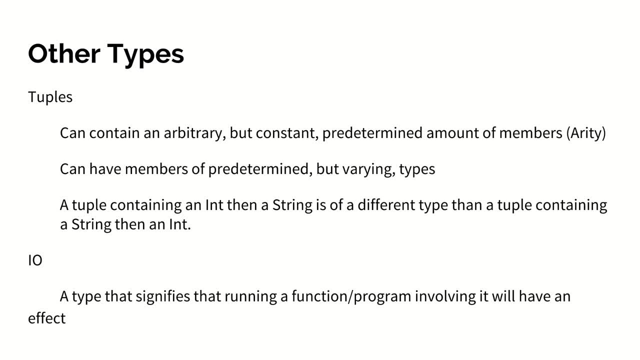 tuple that contains an int, then a string string than an integer. but the tuple may never that same tuple may never contain three integers. Tuples are similar to lists in that the things that they contain actually can determine their true type. A tuple containing three. 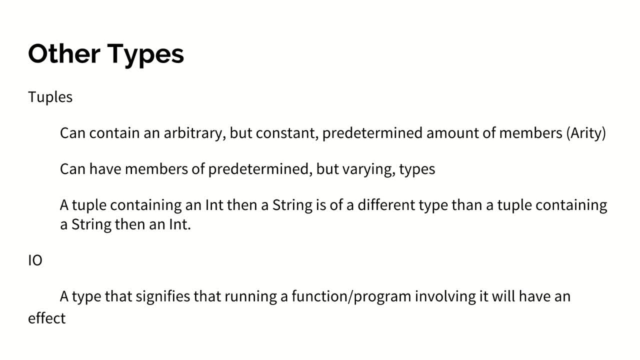 strings is of a different type than a tuple containing three integers, is of a different type of it than a tuple that contains an int, a string and a string. Another common type is IO. This is a type that signifies that running a, running a function or program that involves it will have an effect, but more. 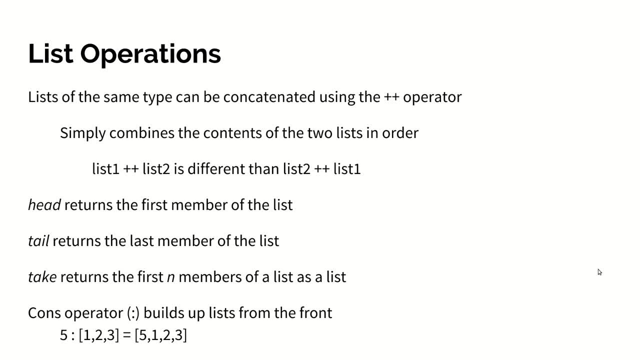 on that in a future video. It's now worth talking about some basic list operations in Haskell. Lists of the same type can be concatenated using the plus plus or concatenation operator, which simply just combines the two lists by putting the contents of the first one in front of the contents of the second one in a new. 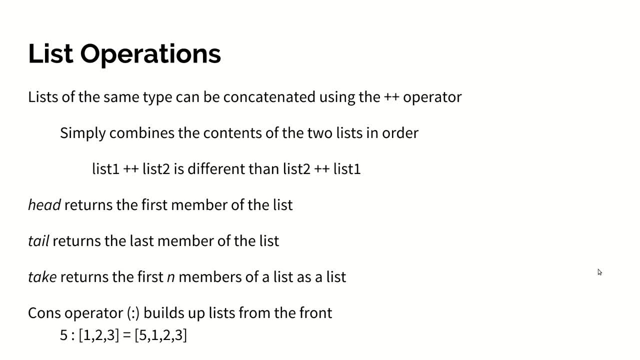 list. The head function returns the first member of the list, tail returns the last member of a list and the take function were returns a sub list. that is the first in members of the list as a list. The Cons operator, which is the semicolon. 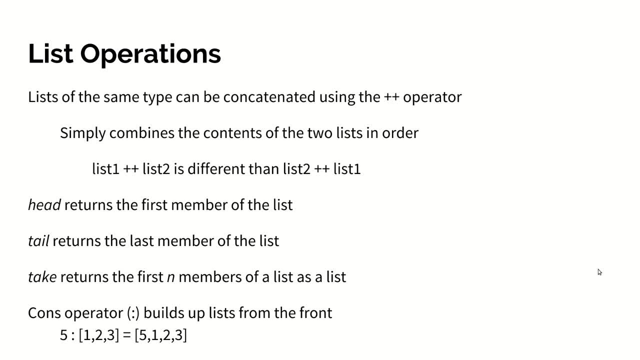 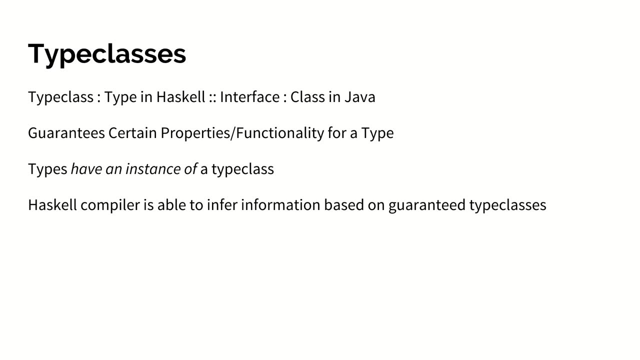 builds up a list from from the front. It's kind of like the push operation. For example, cons one, two, three results in a list of five: one, two, three. So type classes in Haskell are two types, as interfaces are two classes in Java, While this 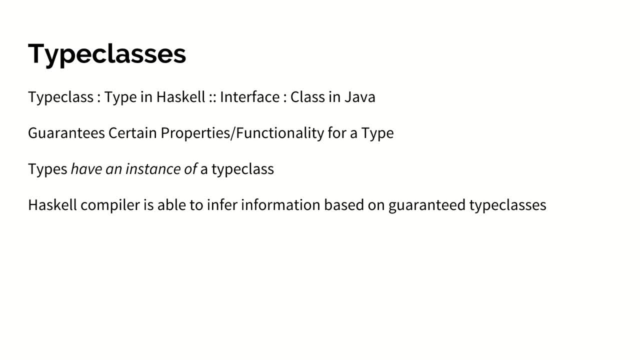 comparison is not 100% accurate to the root principles, it conveys some of the most important information. A type class guarantees certain properties or functionalities about a type. However, we don't really say that types implement a type class. A type has an instance of a type class. Furthermore, the Haskell 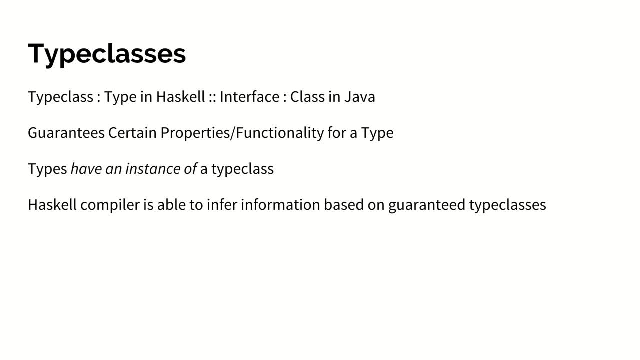 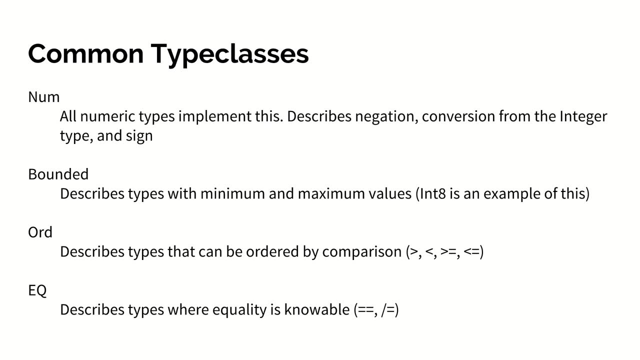 compiler is able to infer information based on type classes that it knows a variable or expression has, but more on that in the next video. Some common type classes include that of num. Num is implemented by all numerals numeric data types. Num describes the ability to negate, convert from the. 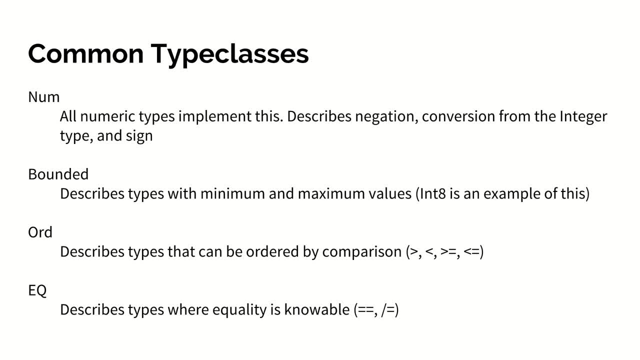 integer type into another type and also get information about the sign of what is described by num. The bounded type class describes types that have a minimum and maximum. For example, int8 has a certain minimum negative value and a maximum positive value because it is limited to a certain number of bits.